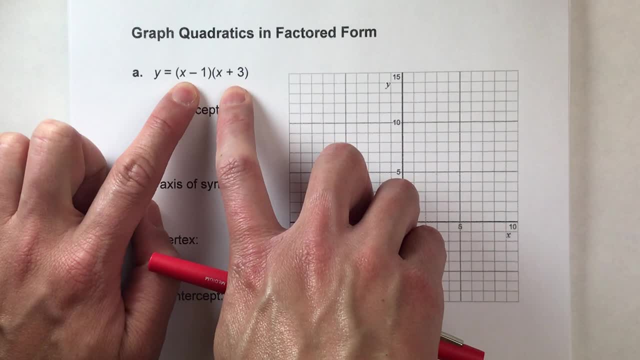 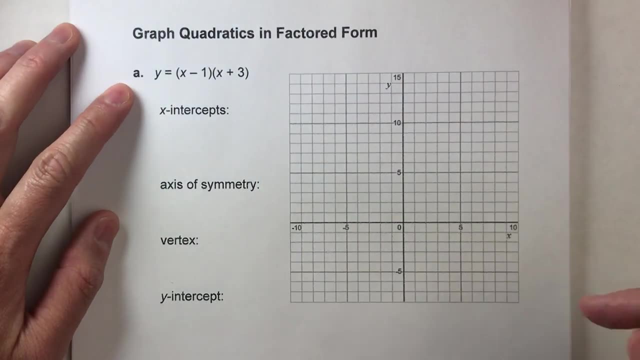 got x minus 1 being multiplied by x plus 3.. Okay, now keep in mind that we know this is a quadratic, so it's going to be a parabola, And because we know the general shape of a parabola and that, 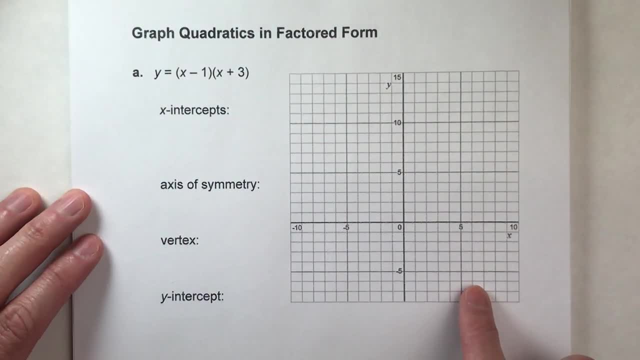 it's symmetrical. we can use that to our advantage when we're graphing. Okay, but we're going to find these four characteristics, these four features of our parabola, and then we're going to use those to graph them. Okay, let's start with the x-intercepts. The x-intercepts are the place. 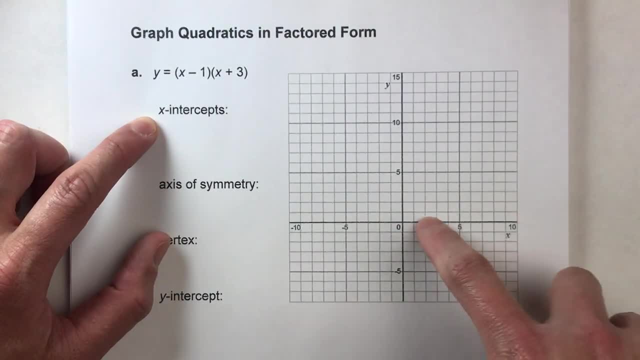 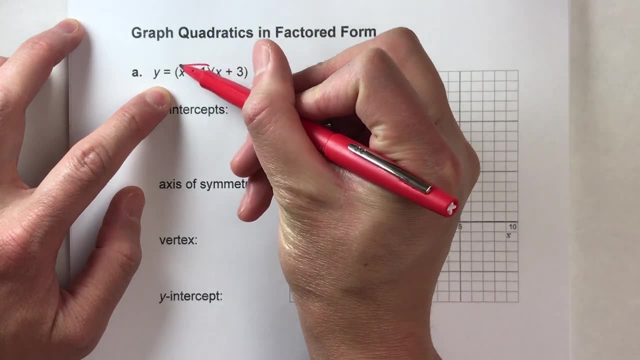 where the parabola crosses the x-axis, and that's when y is zero. All right, so in order to find the x-intercepts from our equation, what we need is for each of the factors to equal zero, And that's going to tell us where the two x-intercepts 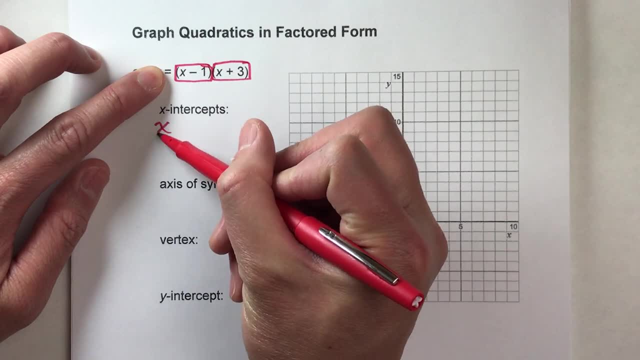 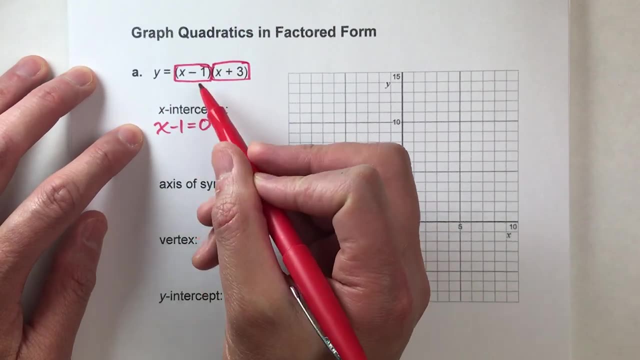 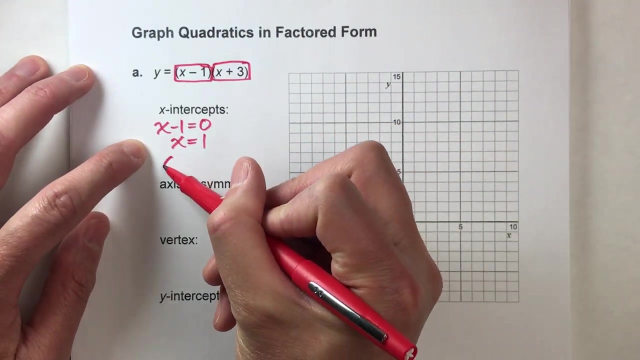 are, For example, in this first factor, x minus 1, we want to know what value of x would make that equal to zero. Okay, if I think of this as a little algebra equation and I add one to both sides, you can clearly see that x has to be 1.. All right, so our x-intercept is 1, 0, right there. 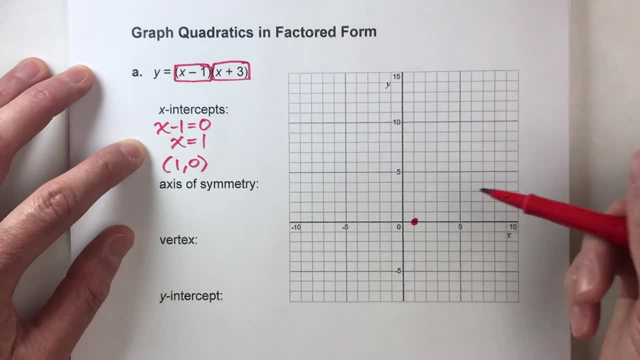 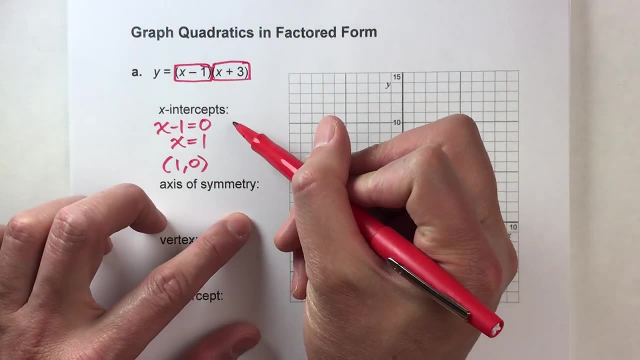 So we know the parabola is going to cross through right there, And if I want the other x-intercept, I'm going to make this other one zero. So in this case, this factor is x plus 3. I'm going to make. 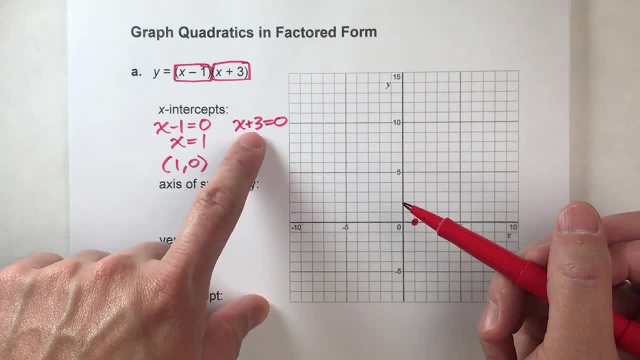 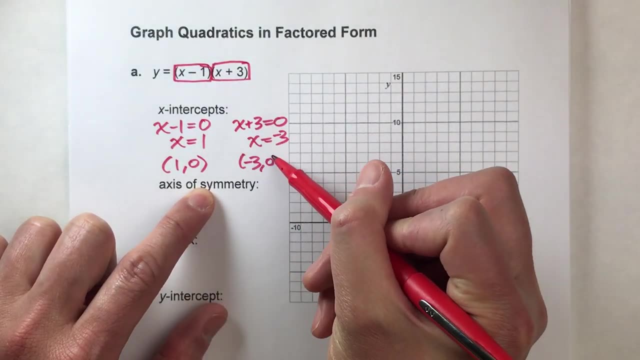 x plus 3 equal to zero. So what value of x would make x plus 3 equal to zero? Well, if we subtract 3 on both sides, we see x is negative 3.. So negative 3, 0 is our other x-intercept. So there we go. 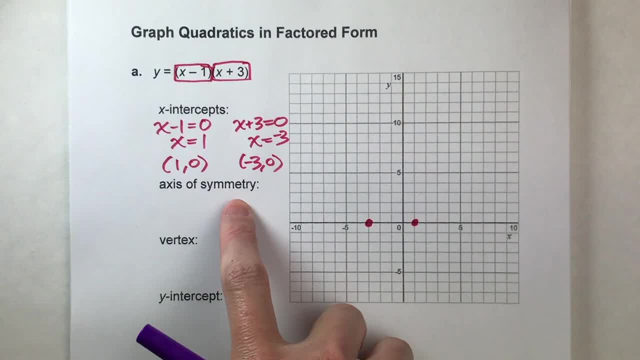 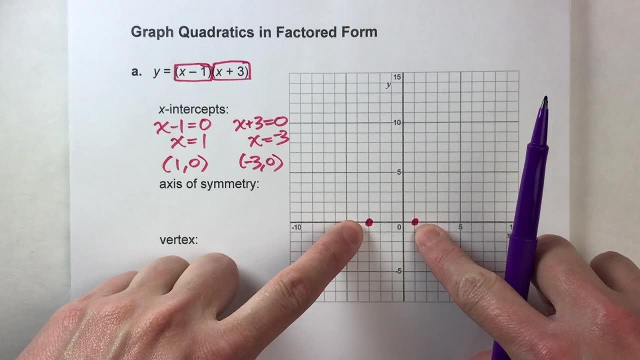 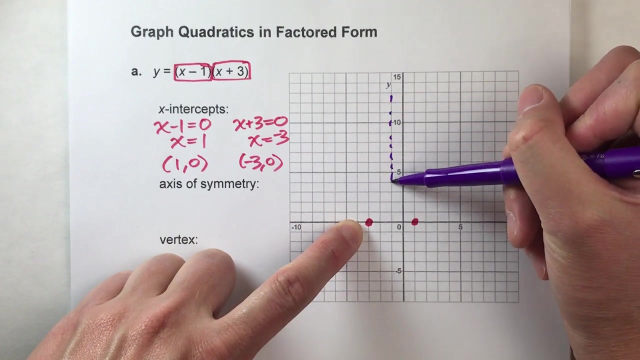 All right. Now the next thing is the axis of symmetry, Because we know a parabola is perfectly symmetrical and we know it's going to go through those two points. we know that the axis of symmetry is going to go right in the middle between them, So it's going to go right through here. 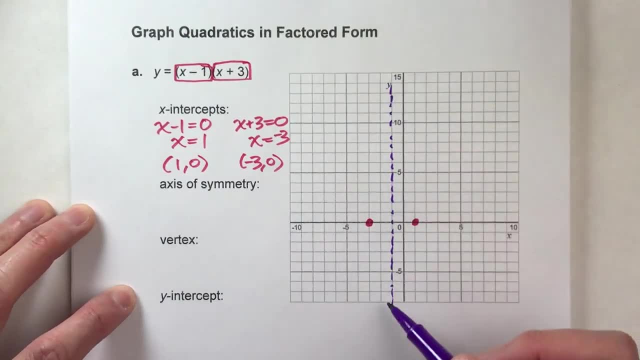 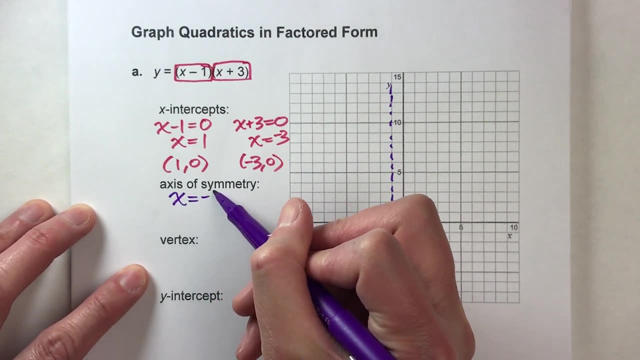 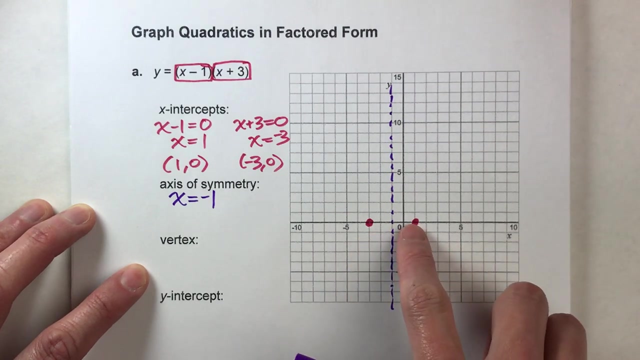 All right, And what is the equation for this vertical line? Well, it's going through. x is negative 1.. So the equation for the axis of symmetry is: x equals negative 1.. It's a vertical line. It's a vertical line through negative 1 on the x-axis. All right, And notice, it goes right in. 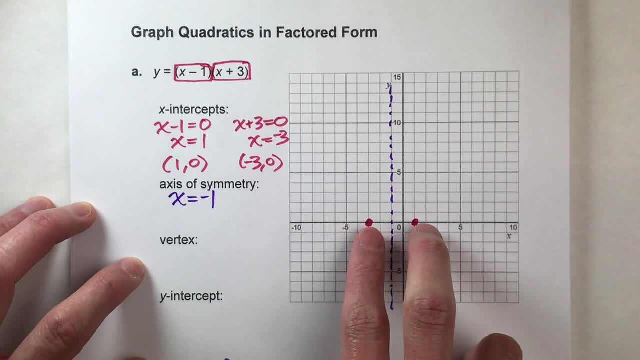 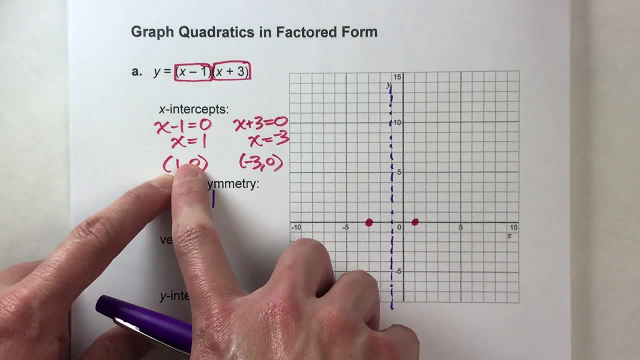 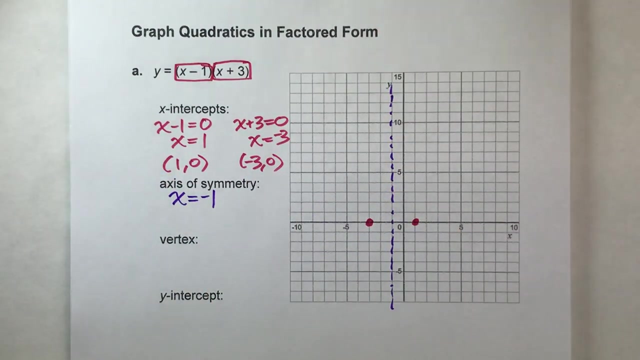 the middle of these two x-intercepts. And if you want to find the axis of symmetry mathematically, all you have to do is take your x-intercepts and find the average right 1 plus negative 3 divided by 2.. You're going to get negative 1, because that's right in the middle of your intercepts. 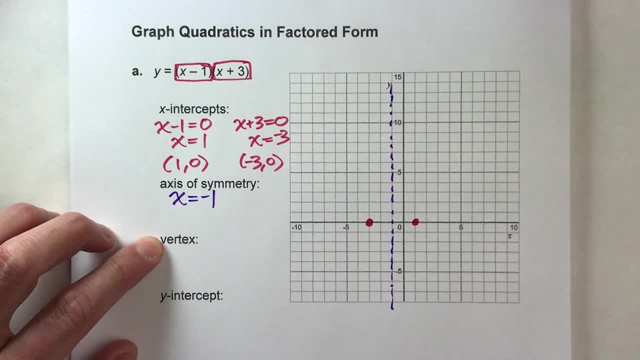 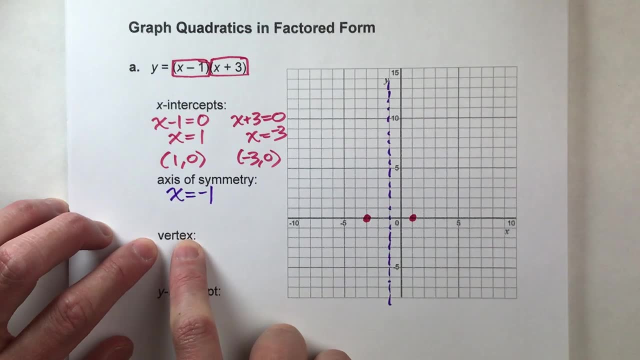 Okay, So now the next thing we need to find is the vertex, Again, because we know the parabola is symmetrical. the vertex is the very tip of the parabola, either the bottom or the top, And because it's symmetrical, we know the vertex is going to be on this axis of symmetry. 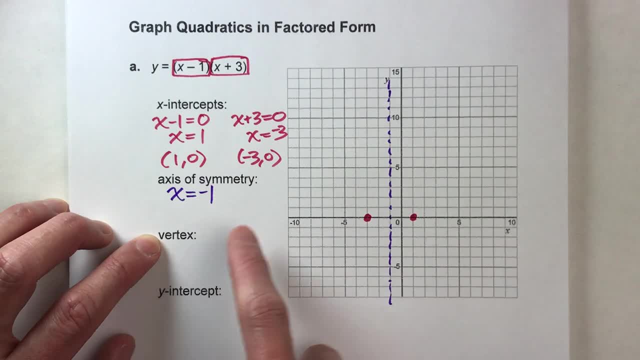 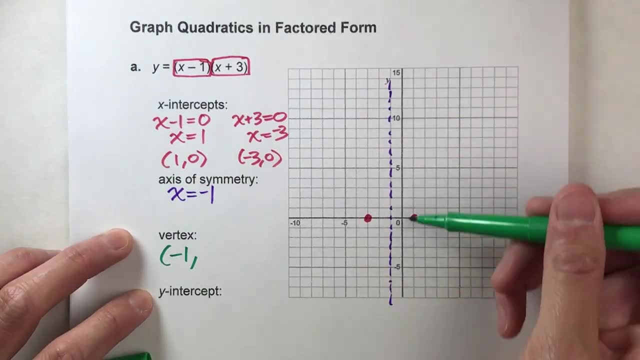 somewhere. All right, So we know the x-coordinate of our vertex, because this line is when x is negative 1.. So we know the vertex is negative 1.. What we don't know is how high up the vertex is going to be. Is it going to be up here? Is it going to be down here? We can figure that out. 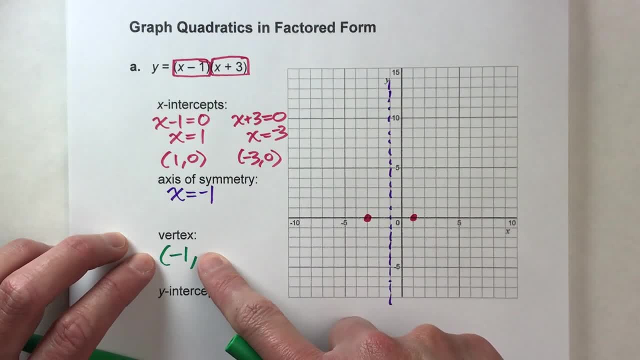 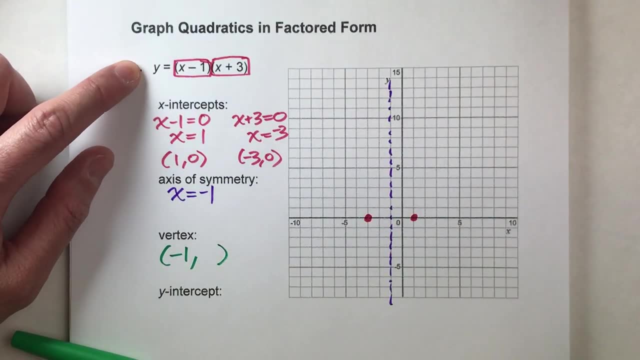 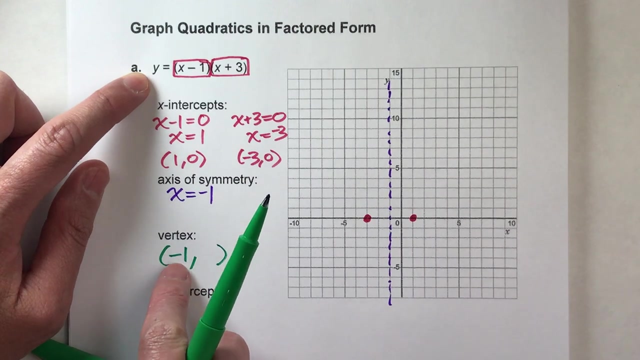 though. Okay, Because we know the x-coordinate of the vertex is negative 1.. What we're trying to find is the y-coordinate. We can use our equation to find the y-coordinate, All right, Because our equation says y equals this. So what we're going to do is take the x-value- we're using negative 1, and put it. 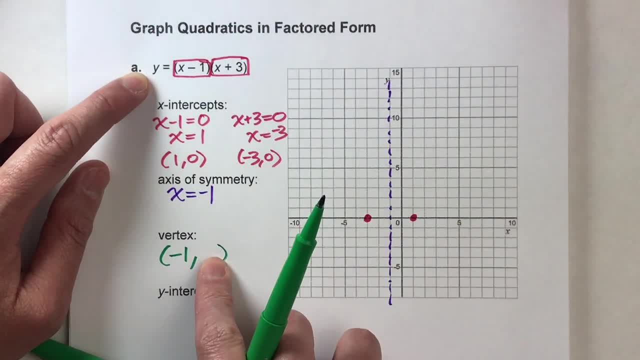 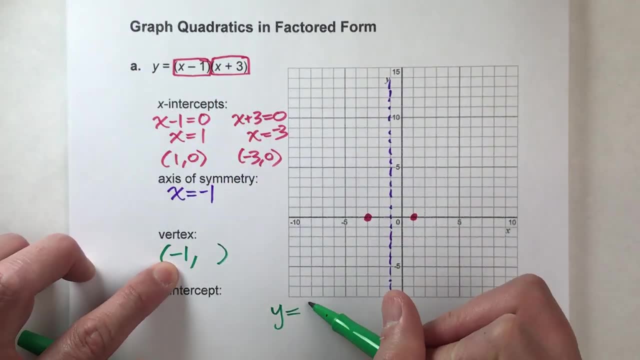 into the equation and that'll tell us the y-coordinate of our vertex. All right, So let me write that down here. y equals: instead of x minus 1, it's going to be negative 1 minus 1.. Times instead of x plus 3, we're going to do negative 1 plus 3.. And whatever all this? 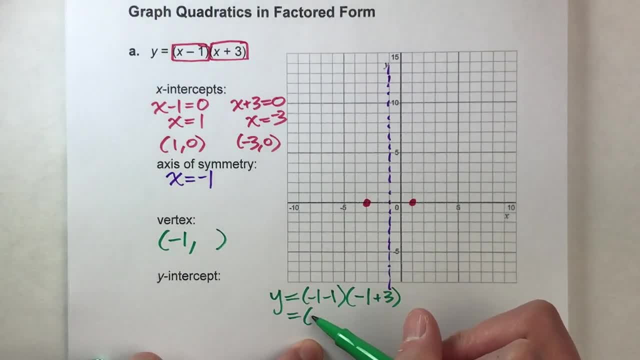 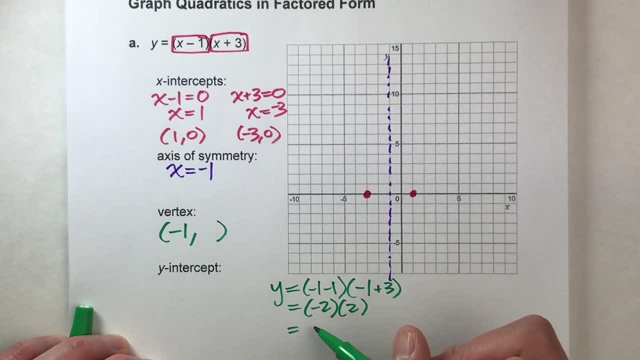 equals is going to be the y-coordinate. Negative 1 minus 1 is negative 2.. Negative 1 plus 3 is positive 2. So y is going to equal negative 4.. We just found the y-coordinate of our vertex. 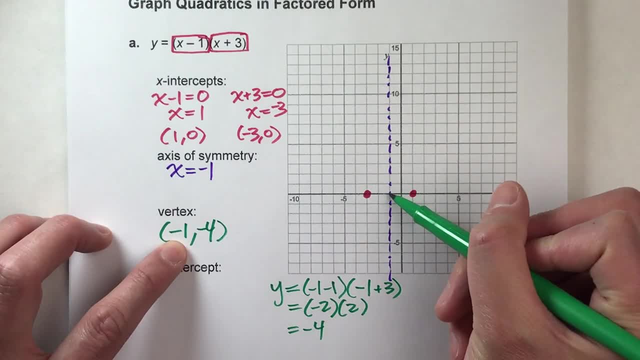 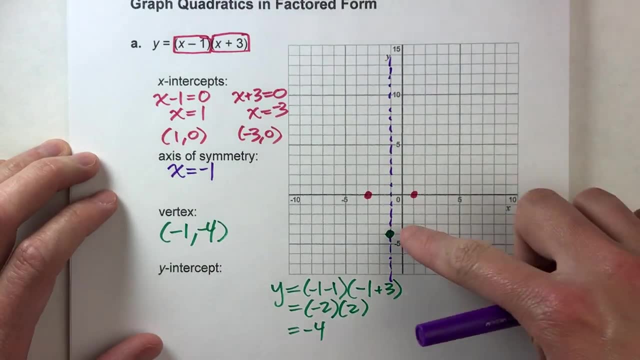 negative 4.. So the vertex is going to be at negative 1, negative 4, right there, All right. And the good thing about parabolas is they kind of follow a basic pattern, So we could actually fill in the rest of it based on this. But we can kind of see what this. 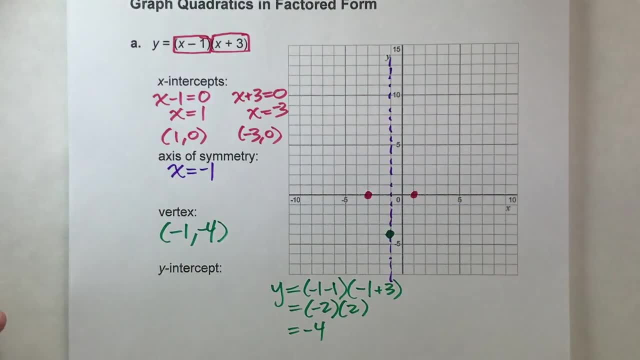 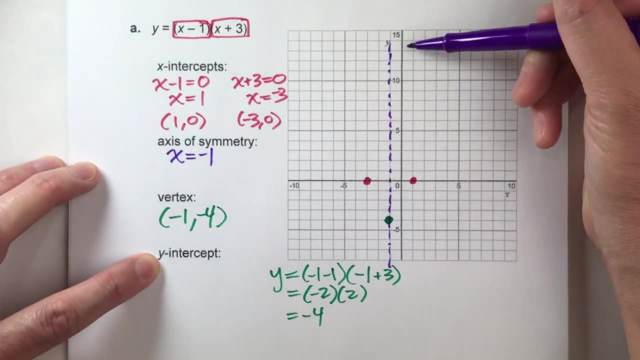 looks like right now. Now you can kind of see the general shape of this parabola. But there's one more thing I want to find and that's the y-intercept. So for the y-intercept it's always going to be on the y-axis. So the coordinates of the y-intercept, because 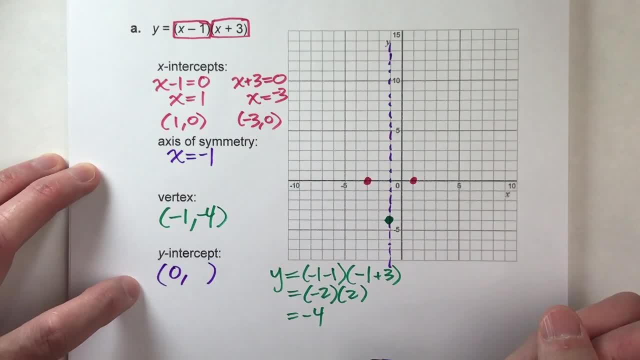 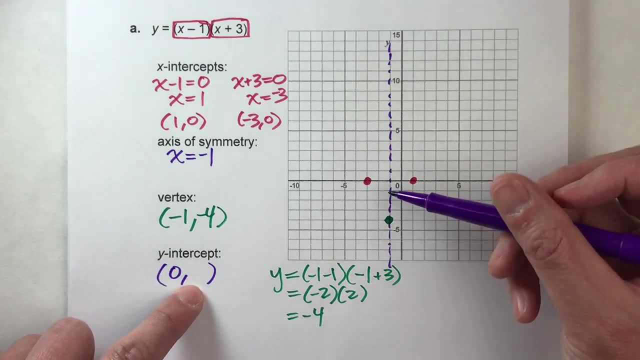 it's on the y-axis, that's when x is 0. So we're going to write negative 1 minus 1, negative 2.. So we automatically know one number in the coordinate. All right, x is 0.. What we? 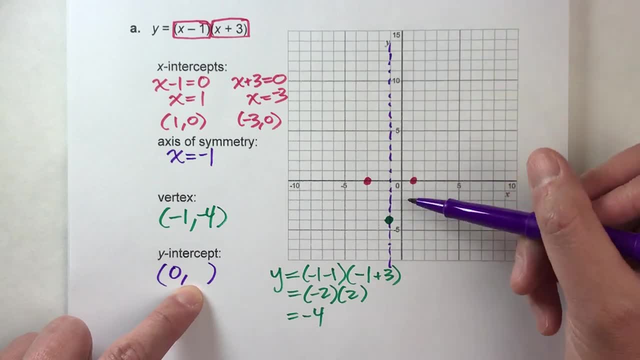 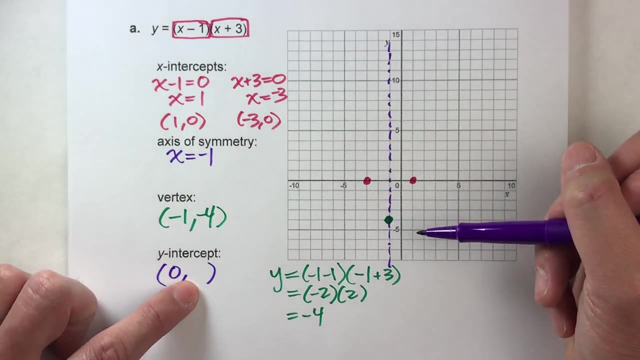 don't know is how high up the y-intercept is going to be, And we know it's going to be in here somewhere, All right. But again, we can use our equation to find the y-coordinate of this point, All right. So what we're going to do is, because we know x is 0, we're going. 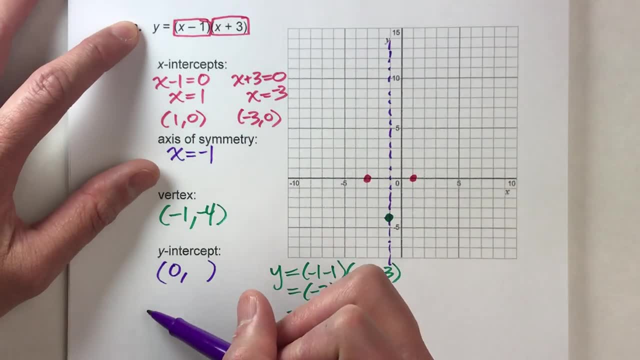 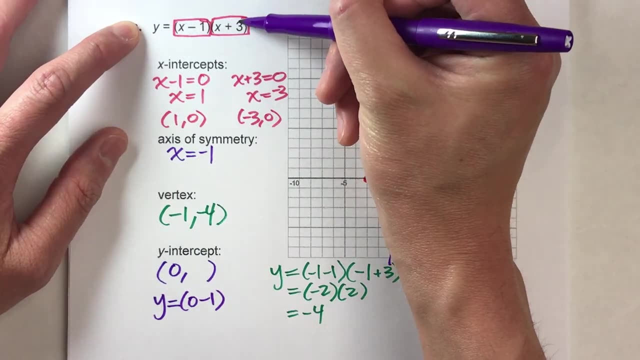 to put 0 in for x in this equation. All right. So y equals: instead of x minus 1, we're going to do 0 minus 1.. Instead of x plus 3, we're going to do 0 plus 3.. And whatever all this, 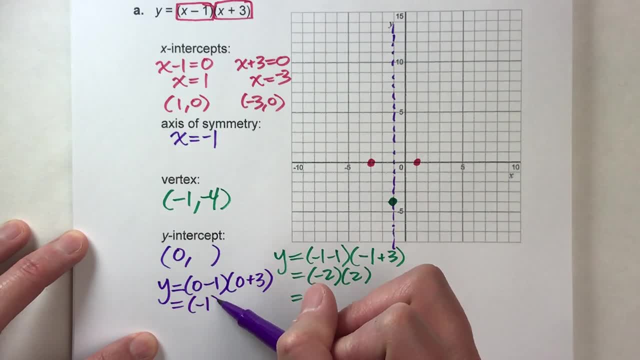 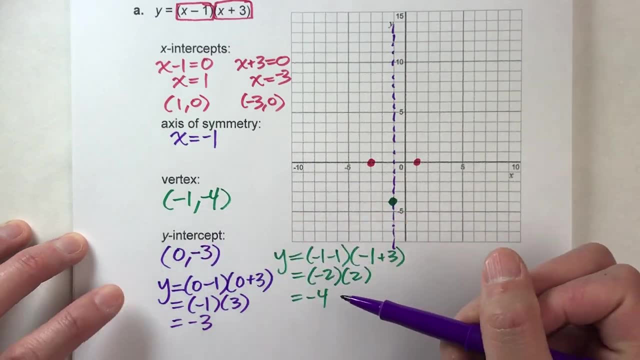 equals is going to be our y-coordinate: 0 minus 1 is negative 1.. 0 plus 3 is 3.. And negative 1 times 3 is negative 3.. Guess what We just found: the y-coordinate of our y-intercept. 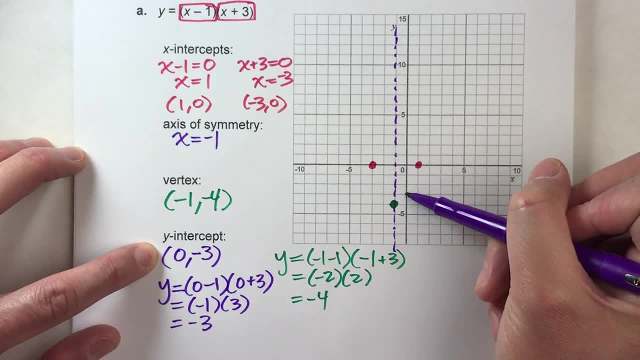 0, negative 3 is the point right there. Okay, And because it's symmetrical, we're going to write negative 1 minus 1.. All right, So we're going to write negative 1 minus 1.. And because it's symmetrical, we're going to write negative 1 minus 1.. All right, So we're going. 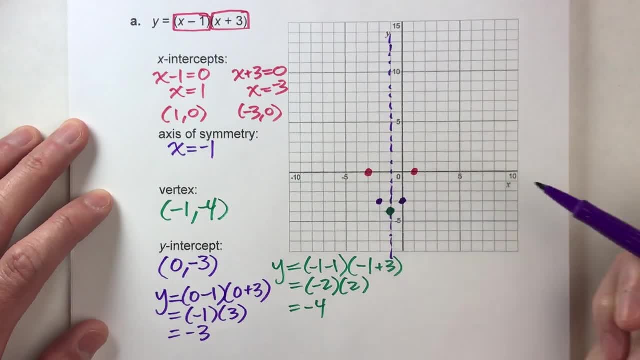 to write negative 1 plus 1.. We are going to write the square root of our term, because x equals 4.. Negative 4 equals 6.. Negative 1 minus 1 equals 7.. Negative 1 minus 1 is negative. 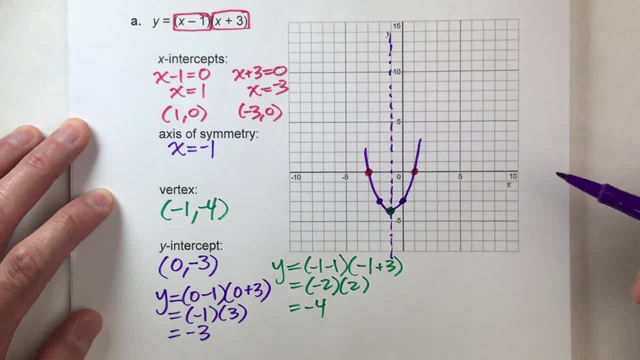 2. Negative 1 equals 6. Negative 3 equals 7.. Negative 6 equals 9.. Negative 1 plus 7 is negative 7.. So we're going to write it down. And of course, now for this y-coordinate. 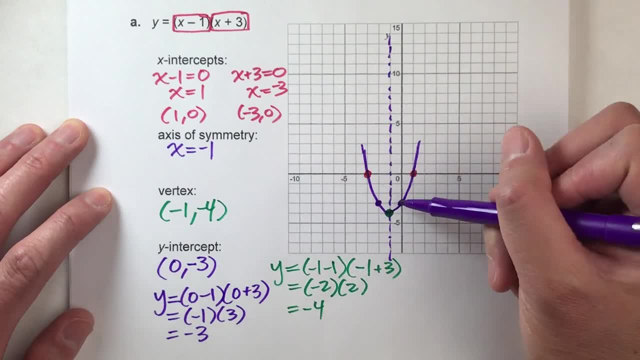 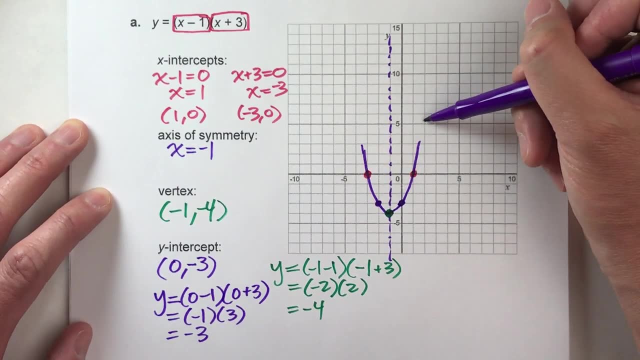 we're going to write our y-intercept Well�. well, we don't have to create a whole fixed set of y-intercepts or an answer table here. So instead, if we worked out that y-intercept, it would have a negative 2 as a whole constructed sage. All right, And we're going to write. 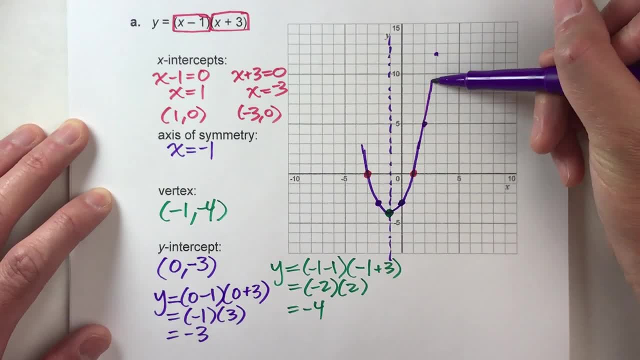 this: negative 1 minus 1 as positive, Not positive. negative 2 times negative, 2 times negative, 5.. So whenever we had a positive nineteen, we're going to write this negative, 2 minus patterns so you can sketch in the rest of it and because it's symmetrical. 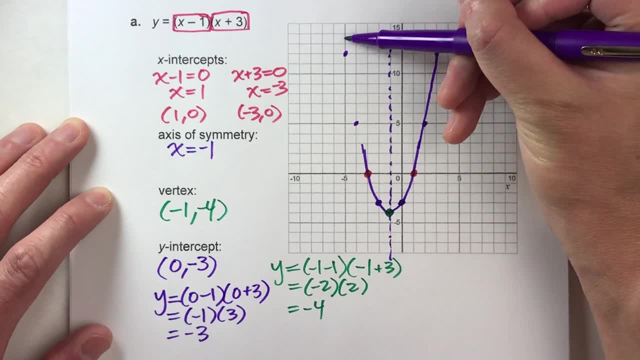 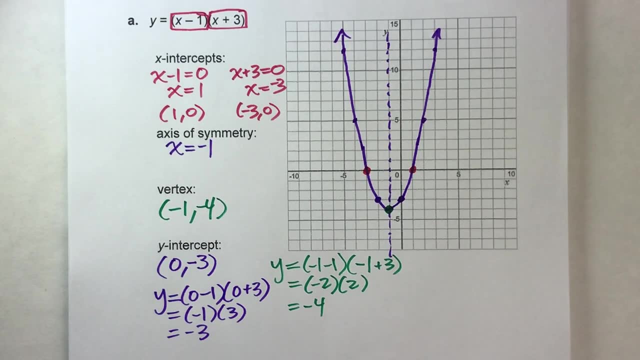 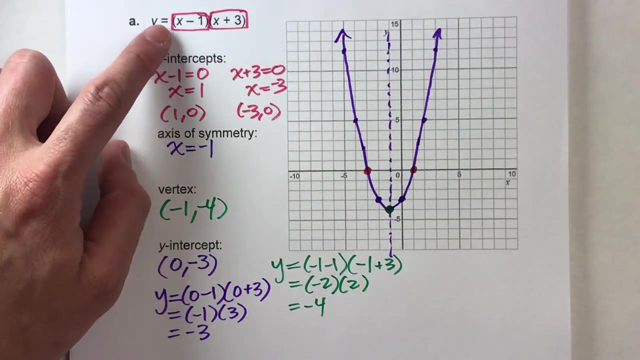 I can just repeat those points on the other side of that axis of symmetry. Alright. so there's our graph, Alright, but let's do another one. that's going to be a little bit harder because, notice, in the factored form, for this one there was no number. 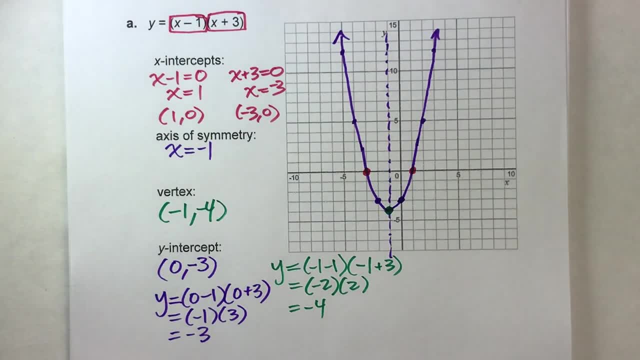 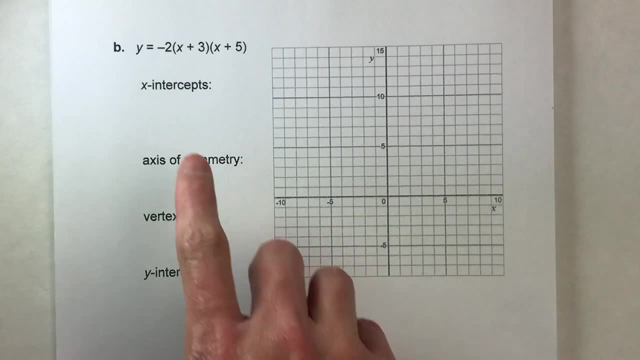 in front of the two factors. The second example is going to have a number there, Alright, so let's pull that one out here. So for our second example, notice, we've got our two factors, but this time we have a number in front of it. 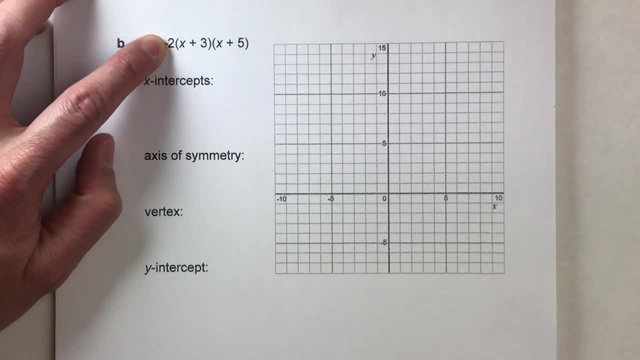 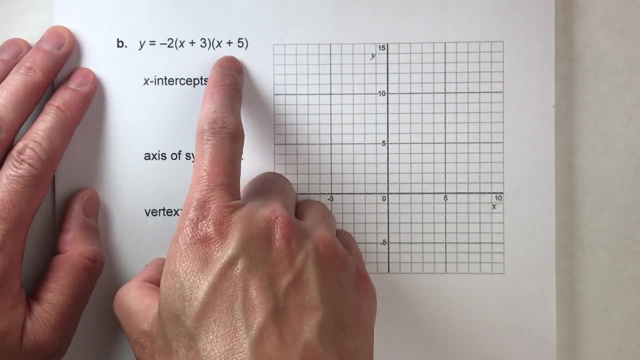 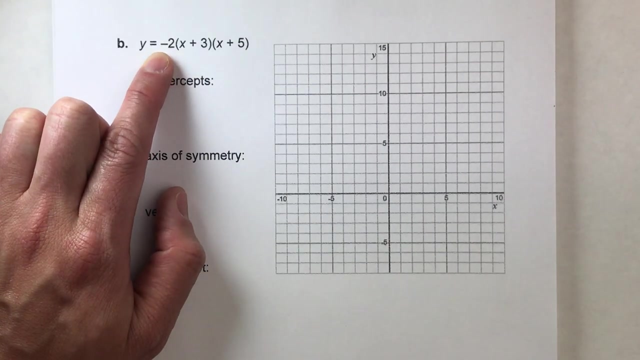 negative two. Now I'll tell you that two is the vertical stretch. It's gonna stretch out our parabola twice as tall as the other parabola we just did. But you see the negative sign That's actually gonna flip our parabola upside down. 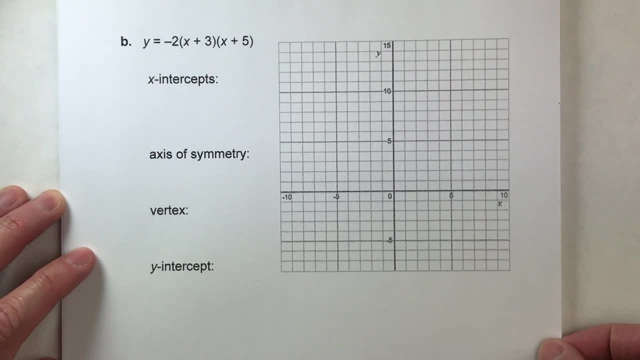 So it's going to be a little bit different than the other parabola we just did, because it's going to be stretched out and it's going to be upside down, But let's go through the same steps because to graph it and find these things, we're 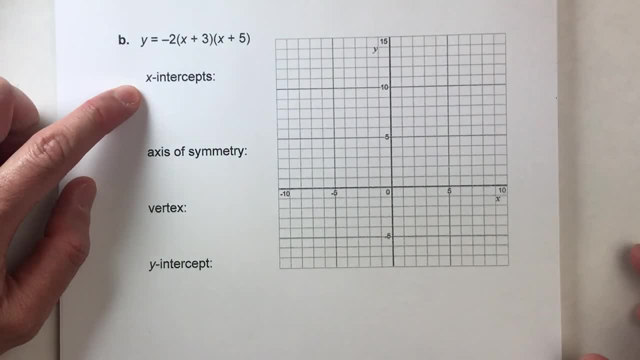 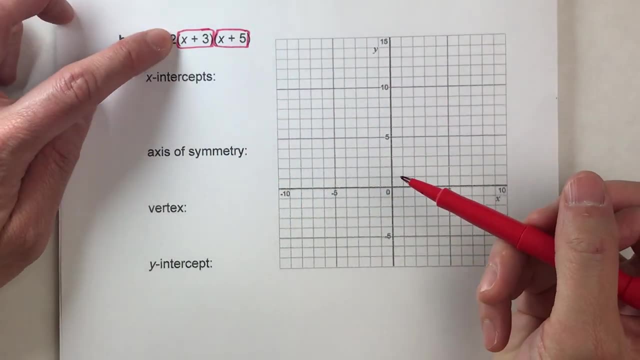 gonna follow the exact same steps. So step one, to find the x-intercepts We need to find when each of the factors is equal to zero. Okay, so when is x plus three equal to zero? Well, that would be when x is negative three. 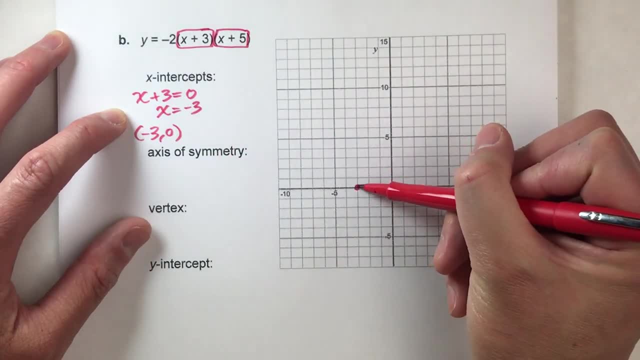 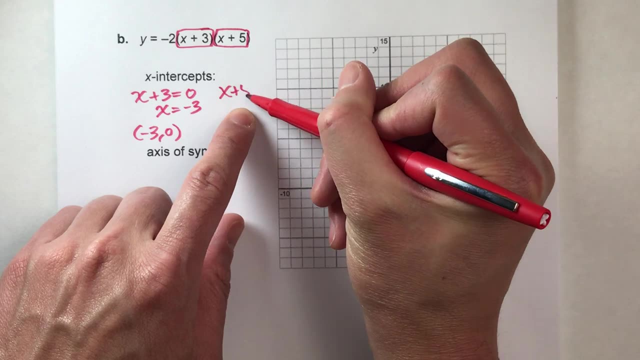 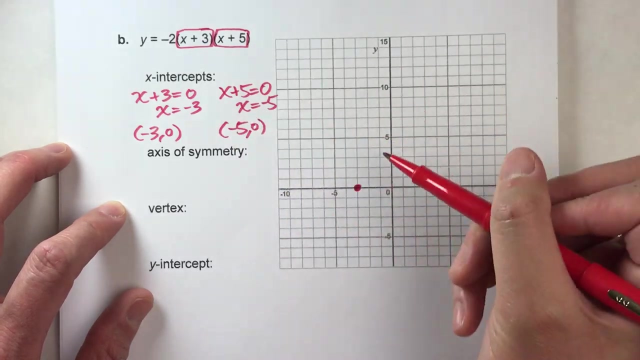 So there is our first intercept: Negative three is zero. Our other intercept is when the other factor is equal to zero. So when is x plus five equal to zero? Well, x would have to be negative five. So negative five, zero is our other intercept. Boom Done. Next thing we need. 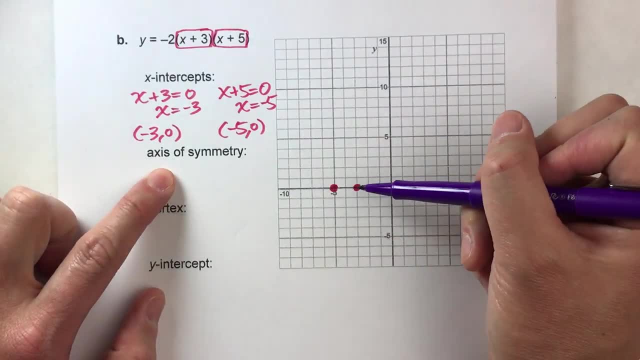 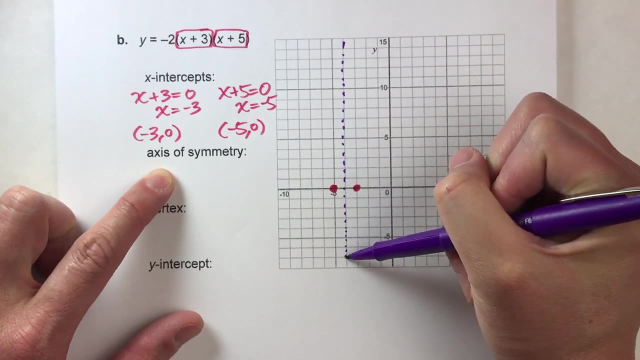 axis of symmetry. Now, remember, the axis of symmetry is going to go right down the middle, right between our two intercepts, So it's going to be right like this: That Boom, And where is that? That crosses the x-axis at negative four and it's a. 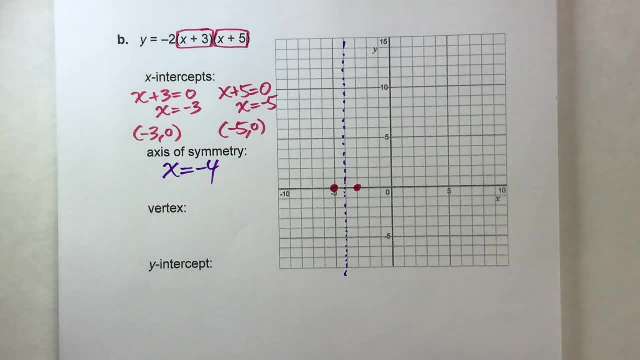 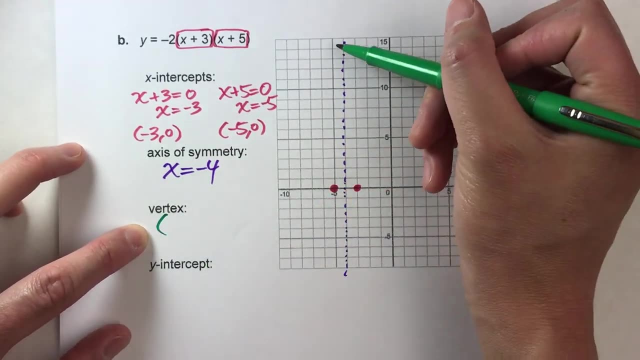 vertical line. So our equation is: x equals negative four. Alright, Next step, The vertex. Now we know the vertex is going to be on this axis of symmetry somewhere. It's probably going to be up here somewhere because, remember, it's upside down. 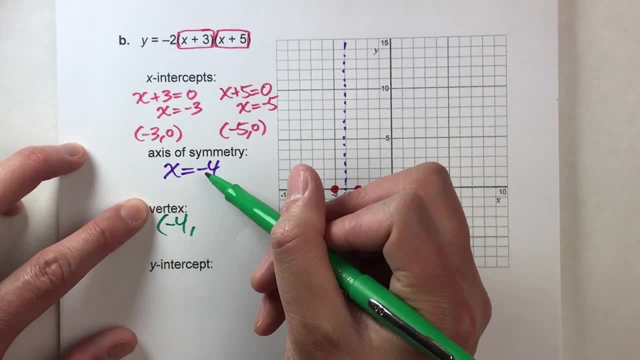 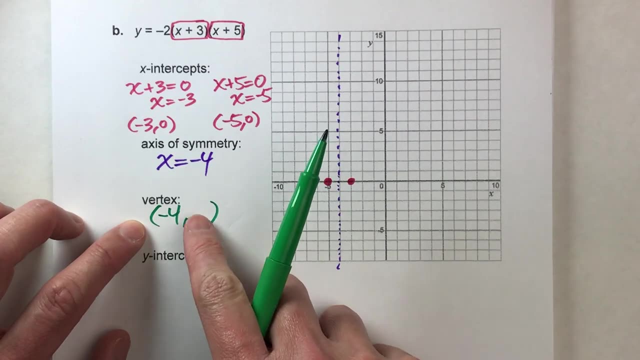 But we know the x-coordinate has to be the same as the axis of symmetry x-coordinate, So it's going to be negative four Something. The only question is: what is the y-coordinate of our vertex? Well, now we can use our equation. 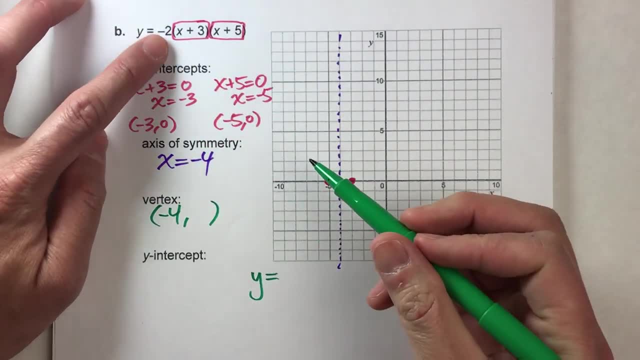 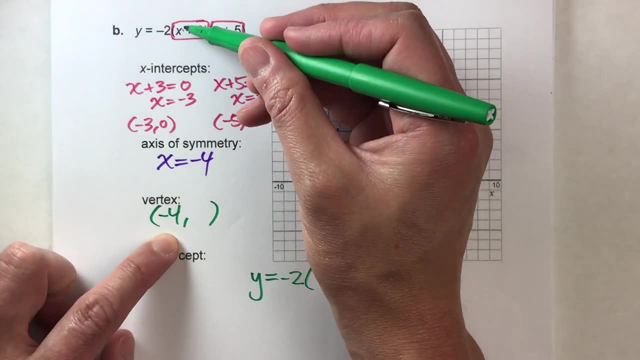 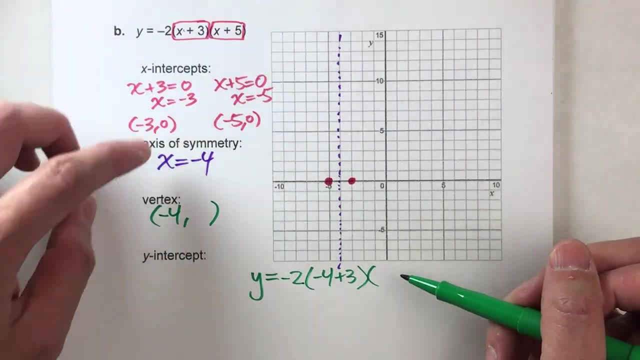 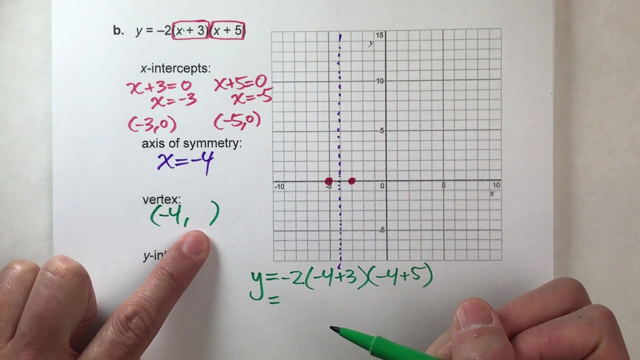 Okay, So y equals negative two times instead of x plus three. We know x is negative four, So we're going to use negative four plus three And times instead of x plus five. we're going to do negative four plus five, And whatever all this equals is going to be the y-coordinate of our vertex. 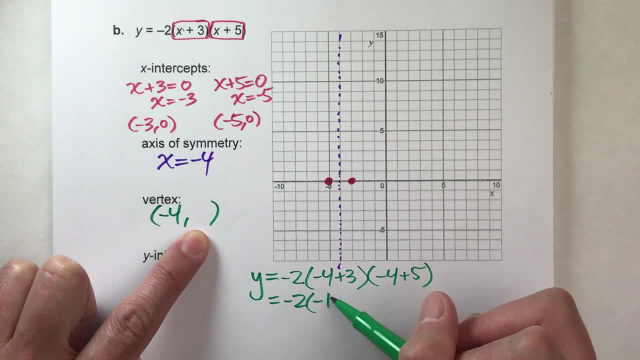 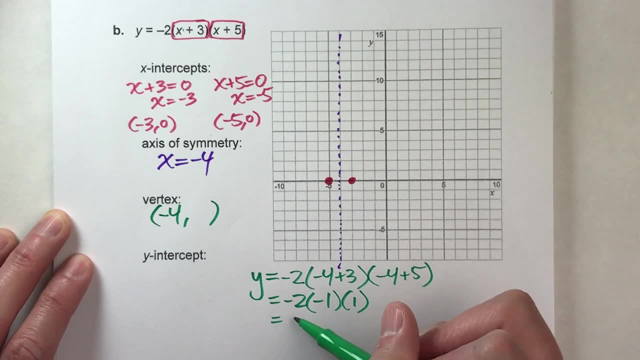 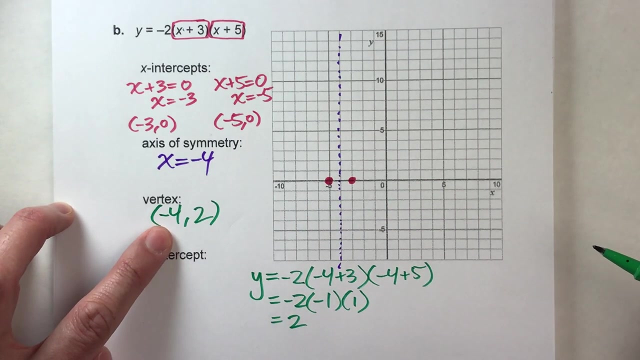 Negative two times negative. four plus three is negative one, And negative four plus five is positive one, And if I multiply this all together I get positive two. So that is the y-coordinate of my vertex: Positive two. So now I know where the vertex of my parabola is: It's negative four. 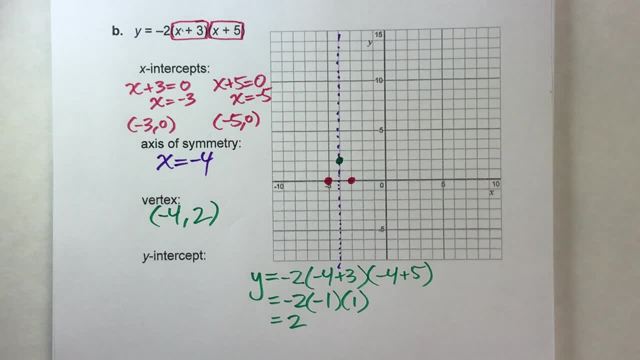 Positive two Right there. That looks good so far, Alright. Now last thing, The y-intercept. Now this one is going to be tricky because, well, we know it's going to be an upside down parabola And you can kind of tell it's already being stretched. 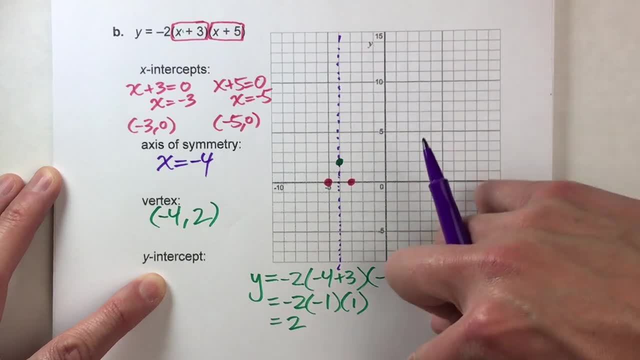 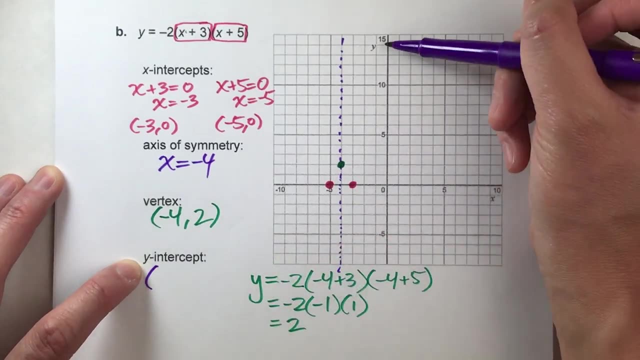 So the y-intercept is going to probably be way down on the y-axis. Alright, But let's figure out what it is. We know it's on the x-axis And it's going to be on the y-axis. So we know the x-coordinate is going to be zero something. 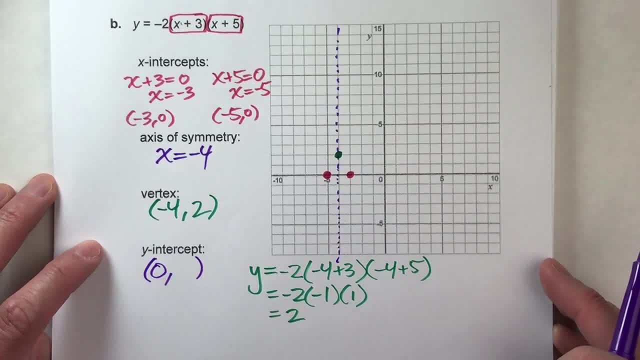 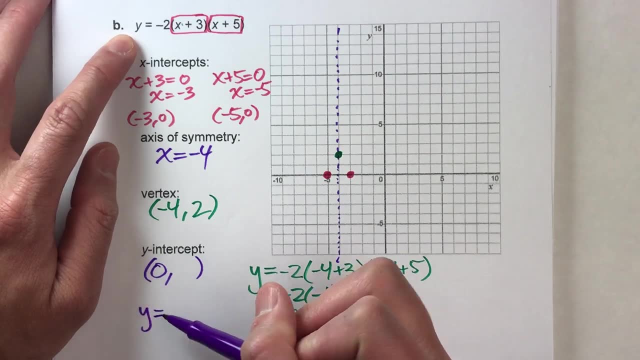 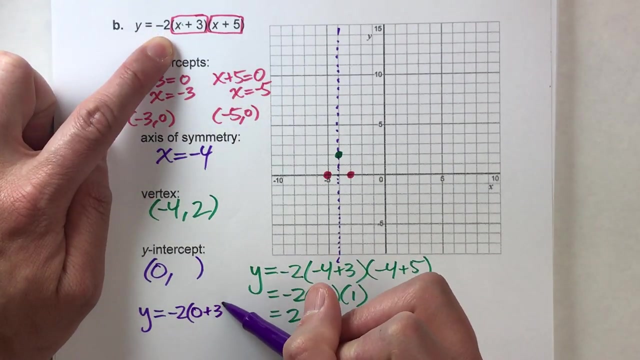 But we don't know the y-coordinate. So let's do this. Let's use our equation to find the y-coordinate. We're going to put zero in for x up there, So y equals negative two times, instead of x plus three, zero plus three. 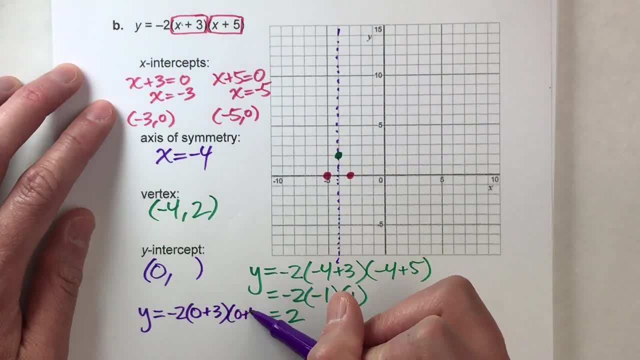 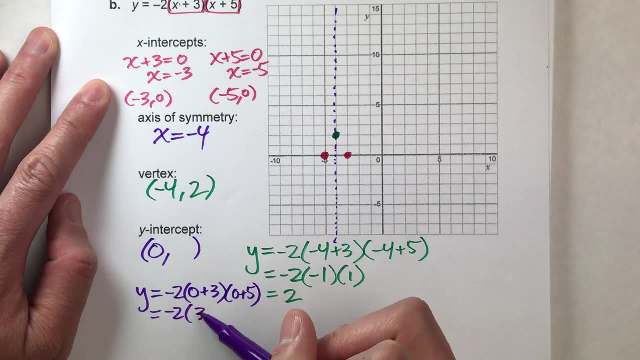 Times instead of x plus five. zero plus five. Alright, So let's see what that equals: Negative two times three times five, Which is going to come out to negative thirty, So that's our y-coordinate. Negative thirty, So there's our y-intercept.